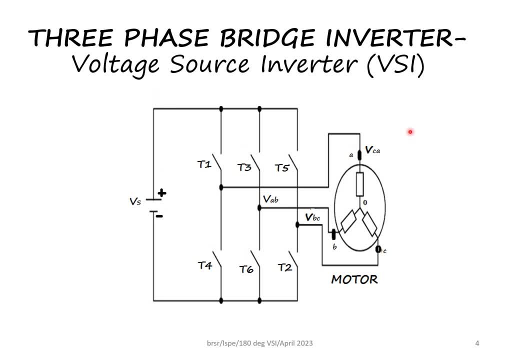 voltage source inverter is given here. This is an inverter operating in 180 degree mode. The input voltage is DC. the output is going to be a AC. three-phase means there will be three waveforms available which are shifted from each other by 120 degrees. Usually the AC output is: 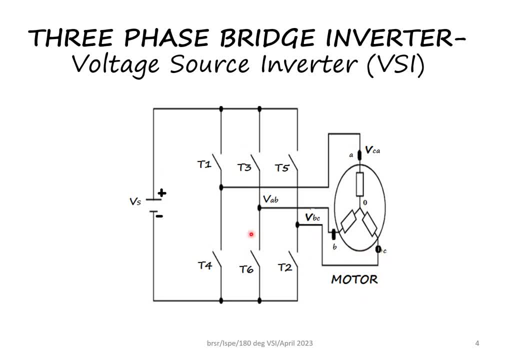 given to a AC motor. Some of the basic things to be understood before understanding the operation of this circuit is: there are six switches available: T1 to TC. The numbering of the switches is given as T1, T3, T5 for the upper group, T4, T6, T2 for the lower. 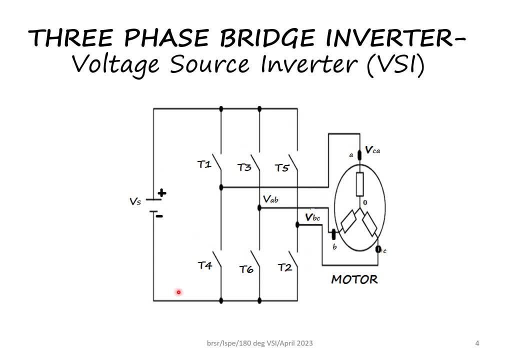 group. It is given like this for the better understanding. and the very first point is: in 180 degree mode of operation each device will conduct for 180 degrees. That means if T1 conducts for 180 degrees, the next 180 degrees T4 will conduct, Then T3 conducts for. 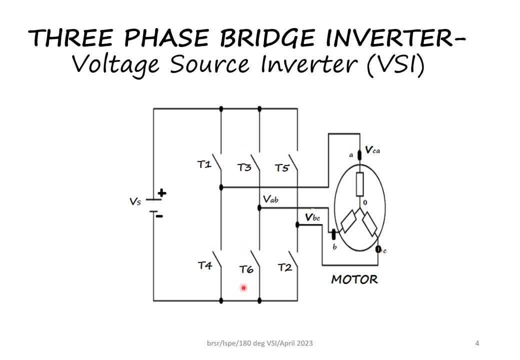 180 degrees. the next 180 degrees, T6. Similarly it is the case for T5 and T2.. In 180 degree mode of operation, at any point of time, three devices will be on. For that a particular sequence is followed If two. 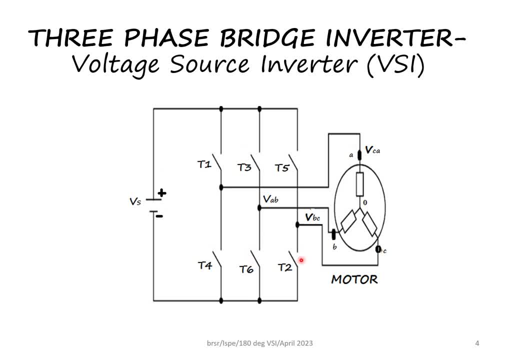 switches from the upper group are conducting, one from the lower group will conduct. If two group, two lower group SDRs are conducting, one from the upper group will conduct. One more important point is the switches in the same leg are not turned on, So the switches 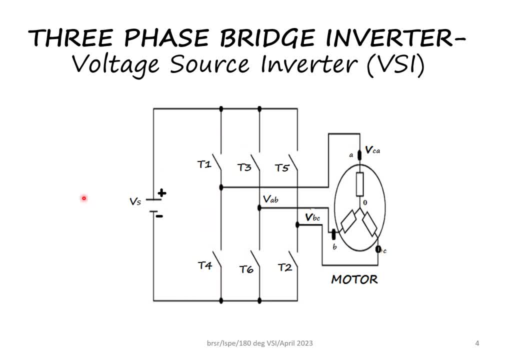 are not turned on at the same time. If they are turned on at the same time, it will give a direct short circuit to the source. So that should be avoided and there is a particular sequence followed for the operation. in 180 degree mode, For example, 561 will conduct. 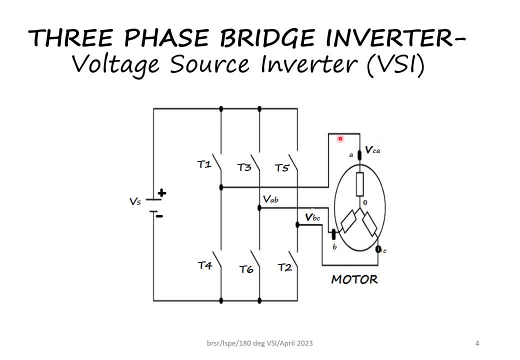 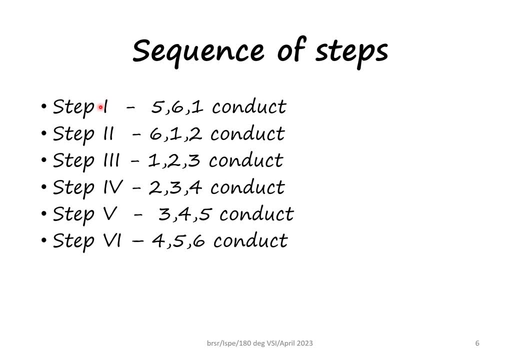 in the very first 60 degrees. Let us see the operation step by step. The sequence of steps is given here. First step, 561 conducts, then 612, then 123, 234, 345, 456.. This is explained in the points. 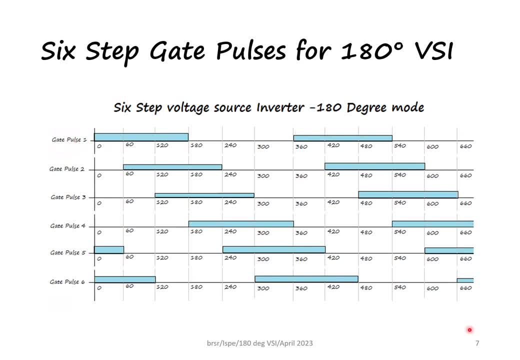 at which the gating pulses are given for the various thyristors, as shown in this image. If the gate pulse is given for a thyristor 1 at 0 degrees, the gate pulse for the thyristor 2 is given at 60,, for 3 at 120,, for 4 at 180, and for 5 at 240.. For thyristor 6, 6,, 6, 6,. 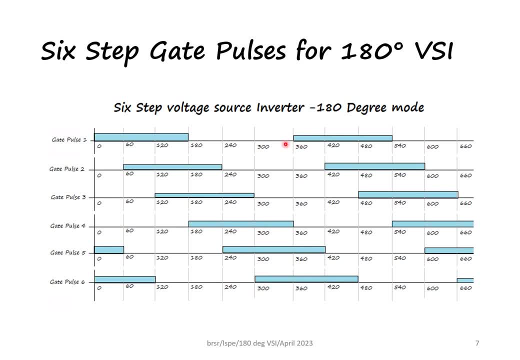 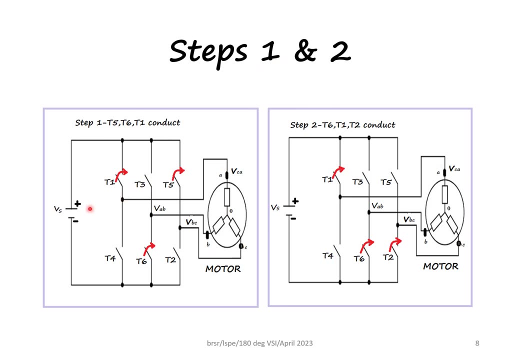 at 300 degrees, Again at 360 degrees the gate pulse for the first thyristor is given. So each thyristor is given the gating pulse at an interval of 60 degrees. Steps like this, steps 1 and 2, is shown here, That is, in the very first 60 degrees 0 to 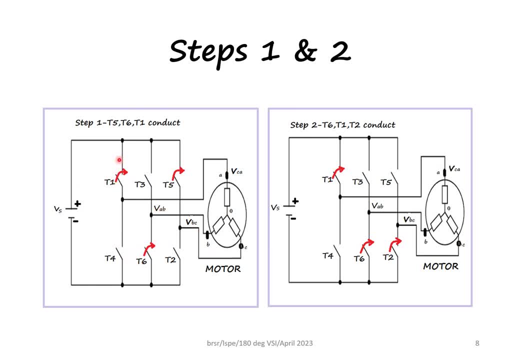 60 degrees of the operation. 3 switches are on. 5,, 6, 1 is on, So 5,, 6, and 1 are shown as Closed. The next operation. this 5 is commutated and 6,, 1, and 2 are conducting The next step. 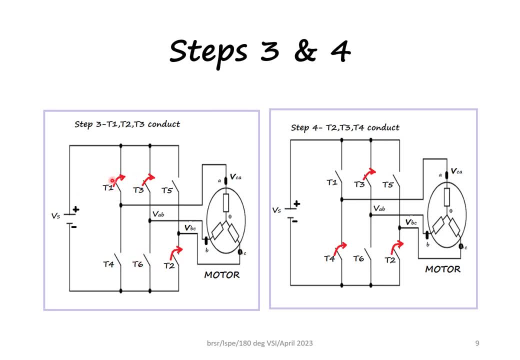 we see that 6 is commutated, 1,, 2, and 3 are conducting And here in the next step we have 2,, 3, 4 conducting. So if you see in any step 2 switches from upper arm and 1. 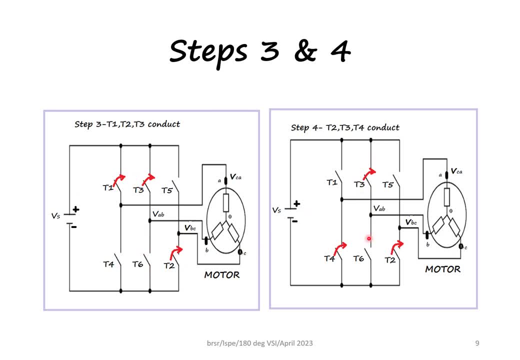 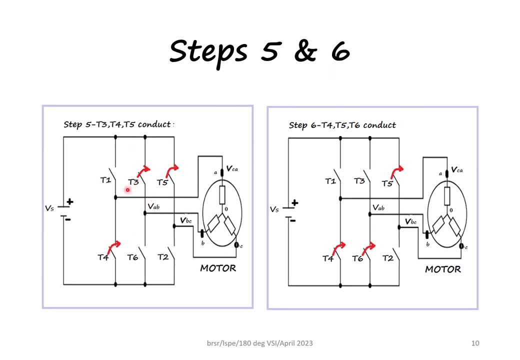 from the lower arm is conducting, Or 1 from the upper and 2 from the lower are conducting. So, similarly, steps 5 and 6 is also shown here: 3 and 5 from upper, 4 from the lower or 2 from the lower. and 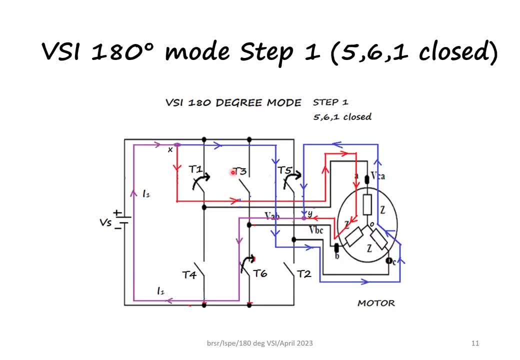 1 from the upper arm, are conducting. Let us see the step 1 operation of the 180 degree mode In step 1, the switches 5, 6, 1 are closed. So here they are shown as closed. switches 5: closed. 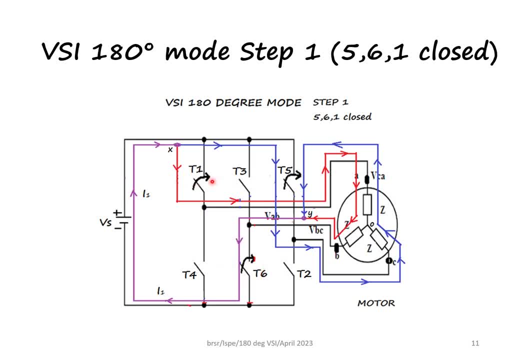 6 closed and 1 is closed. So when the supply is given, the current will flow through these switches. The first path we see here is the current flows from the source, It goes through T1, and it goes through the point A, through the load and goes to B and it comes back. 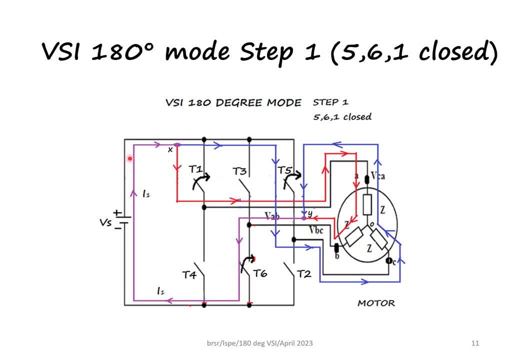 through the switch to the source. So this is the current path, followed by. the switches. 1 and 6 are closed. There is another current path through the switch 5.. Current flows through T5, goes to the load through C and it comes back again. 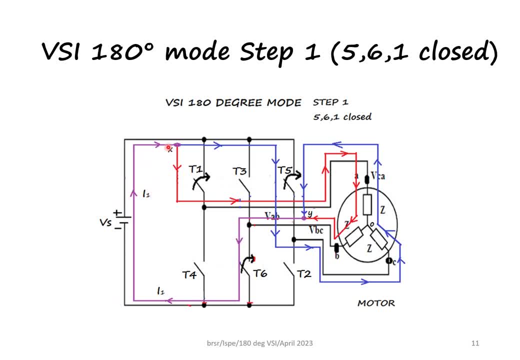 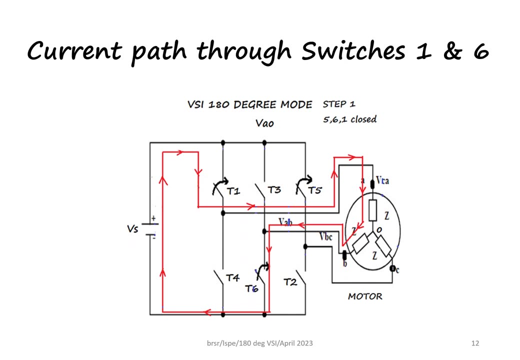 through T6. So we can see that there are two current paths with the total current from the sources I1.. Let us see the operation of this as 1 by 1.. Let us see the current flow through the switches 1 and 6, that is, from the source through the thyristor T1. It goes through the load through. 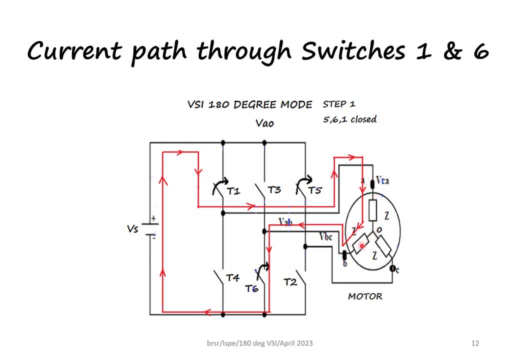 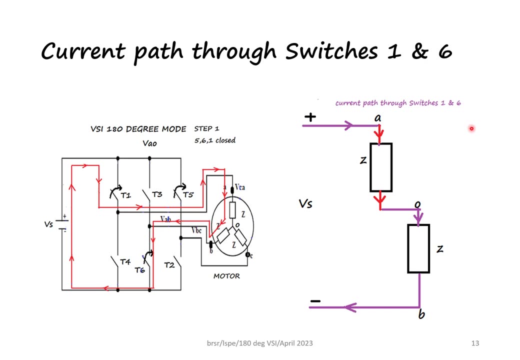 the A, A, O, B and back to the source through T6.. When it is following this path, we can see the equivalent circuit like this: The current is flowing through T1.. It reaches the point A, goes through the impedance. Z goes through this point. 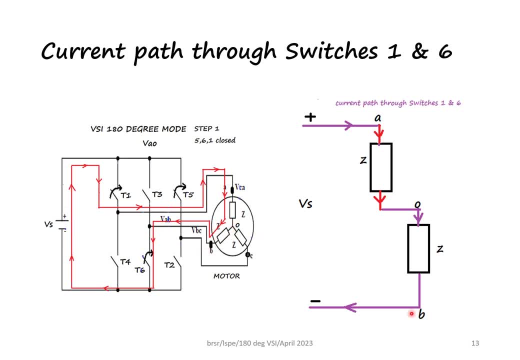 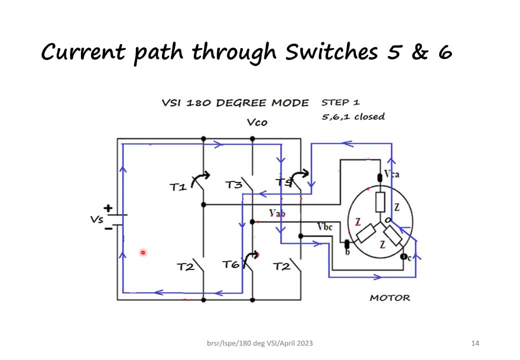 O then goes through the other impedance which is connected to B and it is coming back to the source. If we take the current path through the switch 5, it is from the source through the switch 5.. It goes through the point C, O and it goes back to B. From there it comes like this: 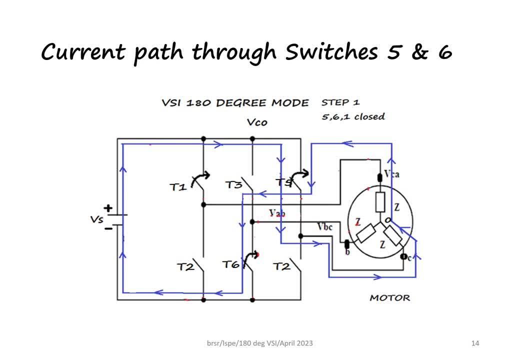 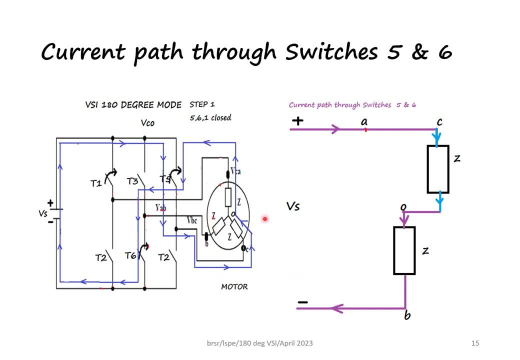 to T6 back to the source. So the equivalent circuit here is: the current is flowing through C- T5. It flows through C O B back to the source. Here it is going through two impedances. The current is getting split into two paths, one in T1, one in T5. Both the switches, when they are. 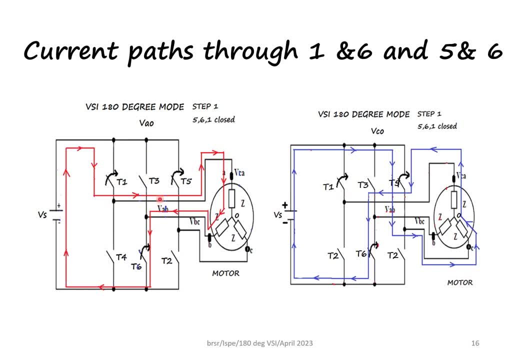 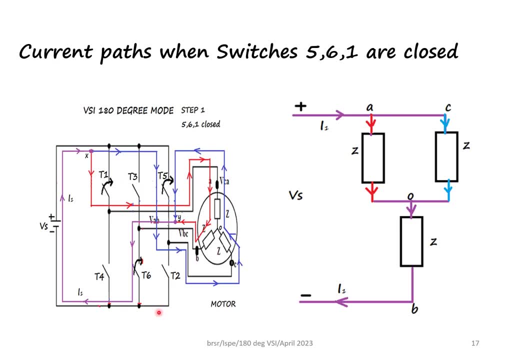 conducting the current paths through 1 and 6 and through 5 and 6 are shown here. So the combined current flow is shown in this picture. So the combined equivalent circuit would be the current flowing from the source to the load will have an equivalent circuit like this. That is the 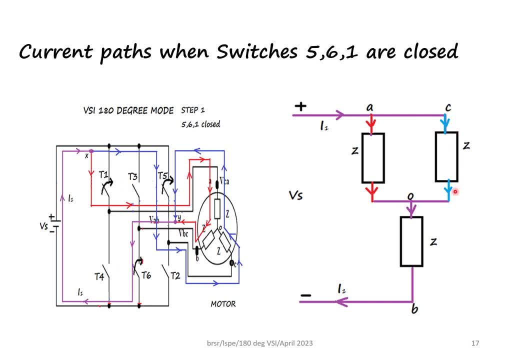 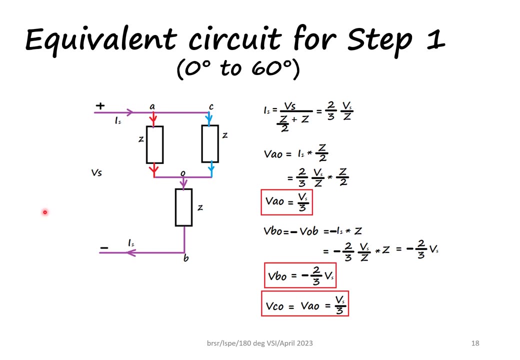 impedance in the A and impedance in the C phase are connected parallel like this, and the impedance in the B phase is connected like this when the switches 5,, 6, 1 are closed. So we can derive an expression for the current as well as the voltages VAO, VBO and VCO for this. 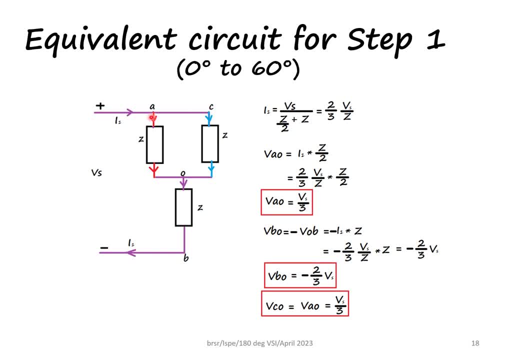 We know that the current flowing is given by the voltage, by the impedance. Here we have two impedances connected in parallel, So the equivalent impedance would be half of it. Two impedances of the same value connected as Z and Z, The total impedance will be Z by 2.. 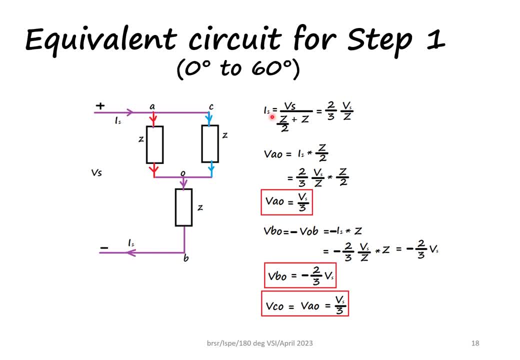 And here it is Z, So the current can be obtained, as current is equal to the voltage, VS divided by the sum of the impedances, Z by 2 plus Z. So that is equivalent to 2 by 3 into VS by Z. This is the. 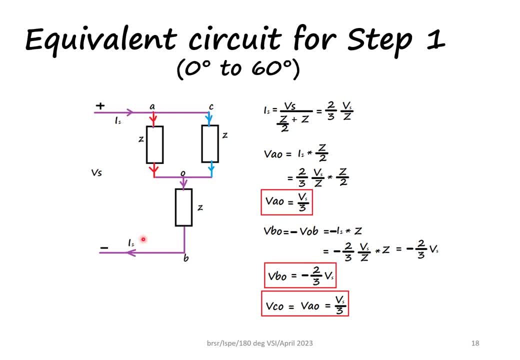 current in the circuit. Let us now find out what is the voltage: VAO, VBO and VCO. Here this total current is split among the three phases, like this: A and C, because they are connected in parallel. they will have a voltage of one-third of the total voltage and this will have the value. 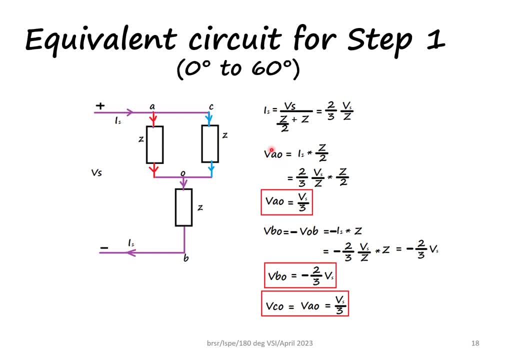 two-third. Here we see that VAO is equivalent to the current into the impedance Z by 2.. That is same for VCO also. So I1 into Z by 2 or I1. we are substituting this value 2 by 3, VS by Z. 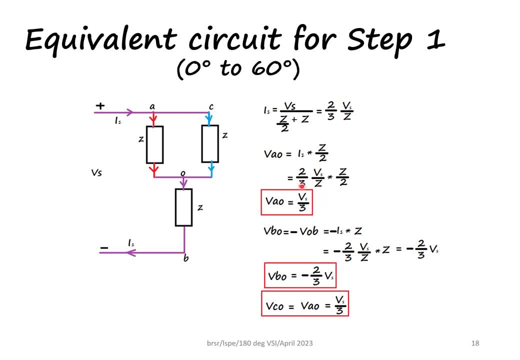 We get VAO as VS by 3. That is, one-third of the source voltage is given for the impedances because they are connected in parallel. like this The balance is two-third of the voltage is available for the other phase, So VBO. similarly, we can write it as minus VOB because the voltage 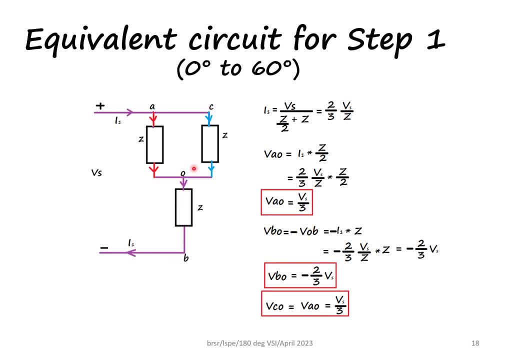 is, we are writing it as VBO but what is available here is VOB. So minus of VOB will be minus of I1.. into the impedance Z, and if we calculate we get this as minus 2 by 3 VZ. So we, if we have, 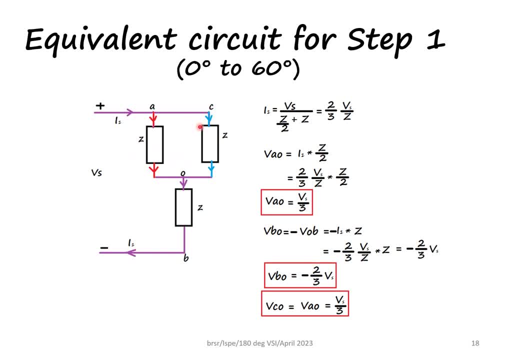 two impedances connected in parallel. they have one-third of the voltage available across it, two-thirds available across the load, So for a period from 0 to 60 degrees. when the steps 5,, 6, 1 are closed, we are seeing the value of VAO, VBO and VCO. The value of VAO- VCO. both are 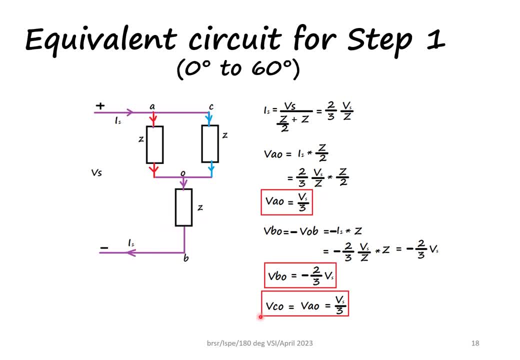 same as one-third of the current. So VBO is equivalent to VCO. So VBO is equivalent to VCO as one-third of VZ Value of VBO is minus of two-thirds of the source voltage. Similarly, for each step we can derive an equivalent value for VAO, VBO, VCO and that can be plotted. 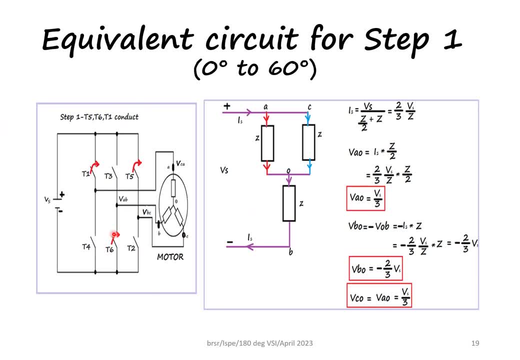 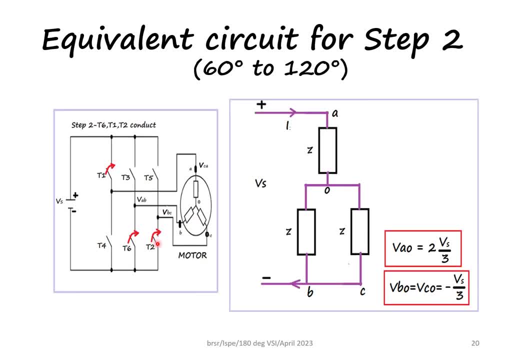 So here this is a consolidated values of VAO, VBO and VCO for the step 1,, that is, 0 to 60 degrees. Similarly, when the switches 6,, 1 and 2 are closed, we can derive an equivalent circuit. 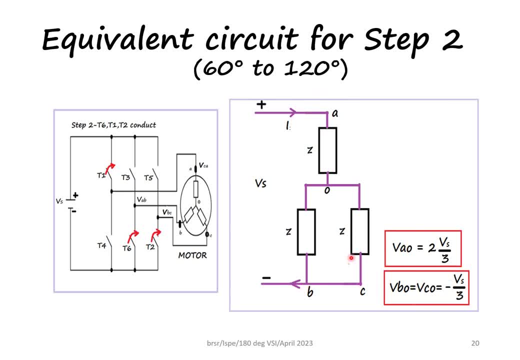 and then find the value of VAO, VBO, VCO. And here, as from the diagram, we can see that VAO should be two-thirds of the source voltage and these should be one-third. and because it is VO, VOC, we are taking VBO, VCO. 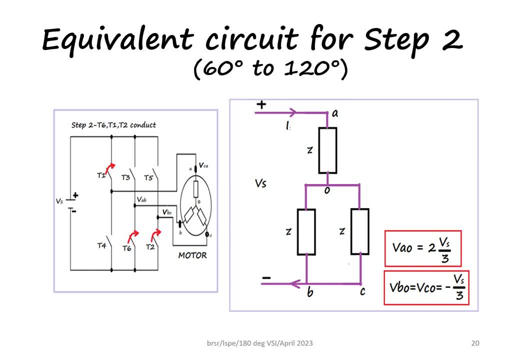 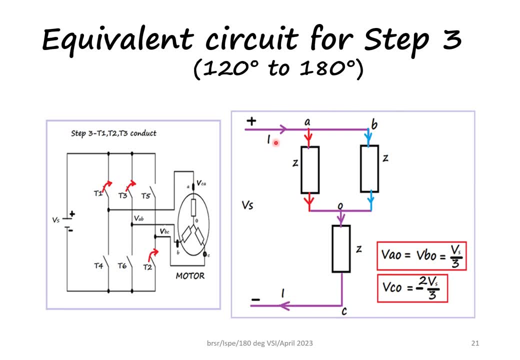 so it should be minus of one-third of the source voltage. Similarly, for the step 3,, 1, 2 and 3 are closed. when we have a equivalent circuit drawn, it will be like this, and here we see that VAO, VPO, both are same and they will be having only one third. 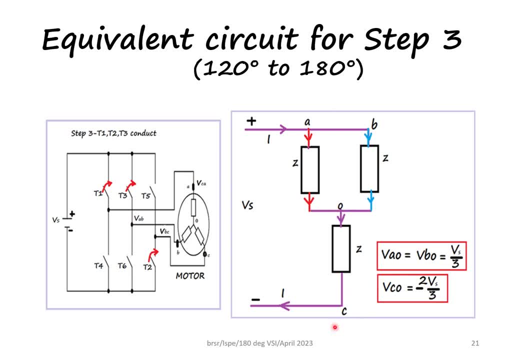 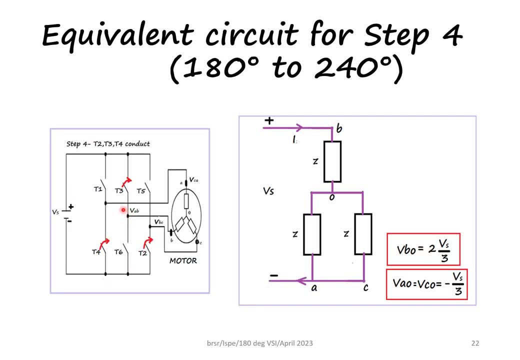 of the source voltage and this VCO is minus VOC and that is minus 2VS by 3, minus two thirds of the source voltage. For the next step, when the switches, that is, 2,, 3,, 4, are closed, we can derive: 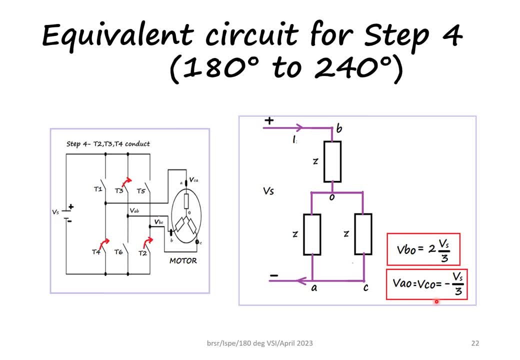 an equation. We can derive an equation for VBO, VAO, VCO like this: because VAO and VCO are connected parallelly and we have the loads connected parallelly, they will have only one third of the voltage, and that too it is in the because it is connected. we are considering VAO. 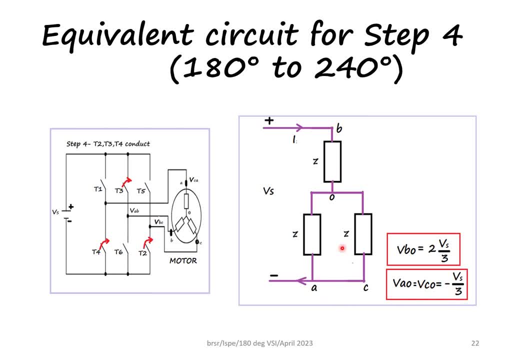 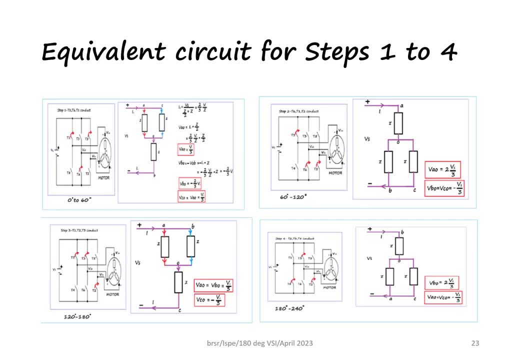 VCO instead of VOA and OC. it is minus VS by 3 and here VBO is two thirds of the source voltage. So for each step we can see like this: we have the circuit, we have the equivalent circuit and we have the values of. 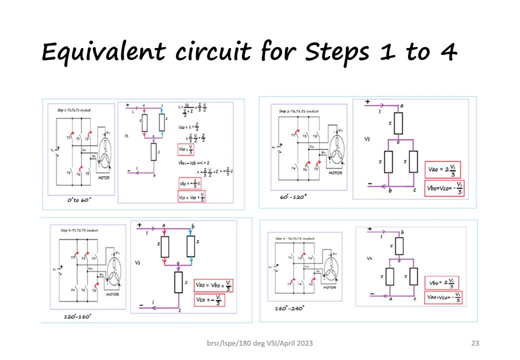 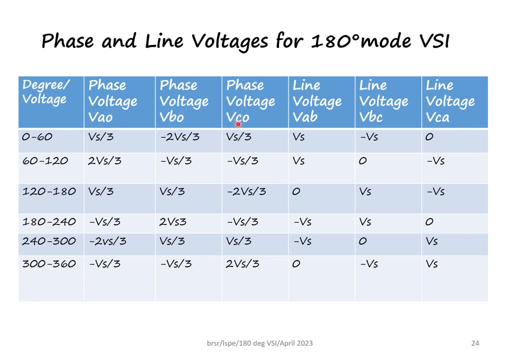 VAO- VBO- VCO for each step. So when we put it in a table like this, VAO- VBO- VCO, we get VS by 3, 2VS by 3, VS by 3 and the repetition as minus VS by 3, minus 2VS by 3, minus VS by 3.. 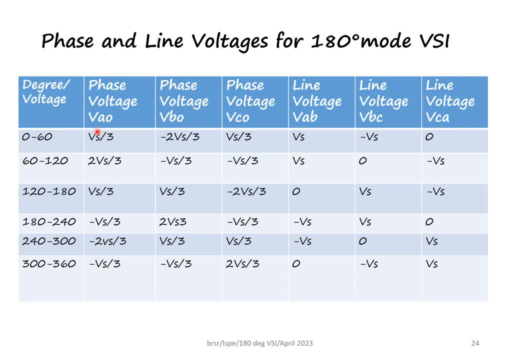 For each step, it is like this. So, for each step, it is like this. So, for each step, it is like this. To remember it better: VAO is starting at 0 to 60 degrees, as VS by 3, VBO will be starting at 120. 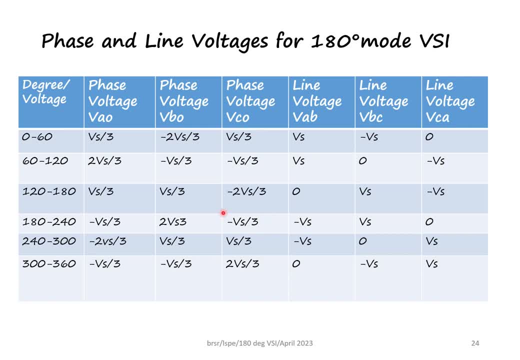 degrees as VS by 3,. VCO will be starting at 240 degrees as VS by 3.. The sequence followed is: VS by 3,, 2VS by 3, VS by 3,, minus VS by 3,, minus 2VS by 3 and minus VS by 3 to. 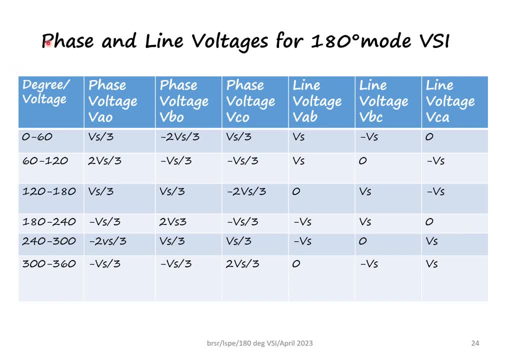 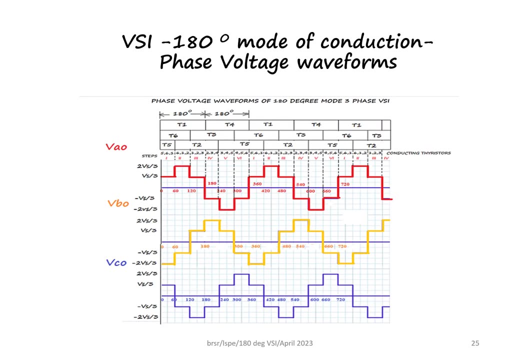 write the values in a table like this. It is easier to remember this way and when it goes to, when this is plotted in the waveform, it will look. when the values derived in the table are plotted in the graph, we can see that VAO is starting as. 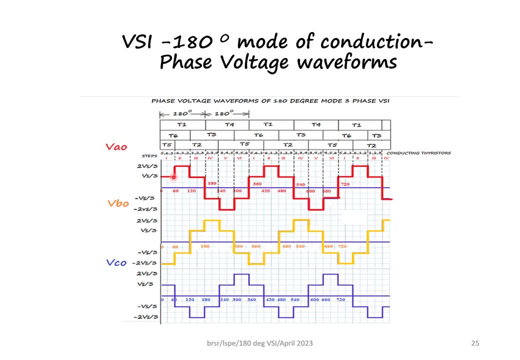 VS by 3 at 0, then the value of VS by 3 has become 2VS by 3 at 60 to 120 interval and it is again becoming VS by 3.. We have derived these values in each step, The very first step. we have seen that. 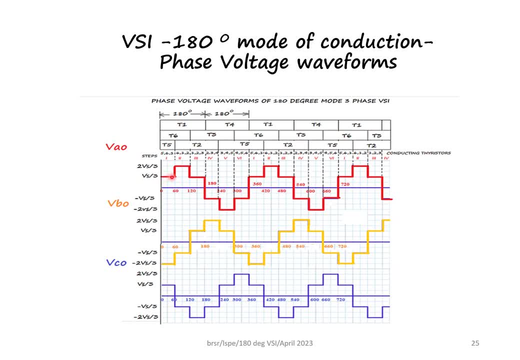 VAO and VCO in the interval 0 to 60 degrees had a value of VS by 3 and VS by 3. here VBO had a value of minus 2VS by 3, which is shown here. So for each step from the table, if it is, 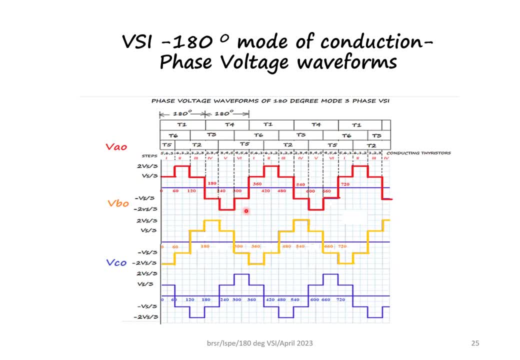 plotted, we get a pattern like this and we can see that VAO is starting at 0, with VS by 3 and following a pattern. VBO has the same pattern but it starts at 120 degrees and VCO also has the same pattern, but starting at 240 degrees. These values- VAO, VBO, VCO- are all the phase values. 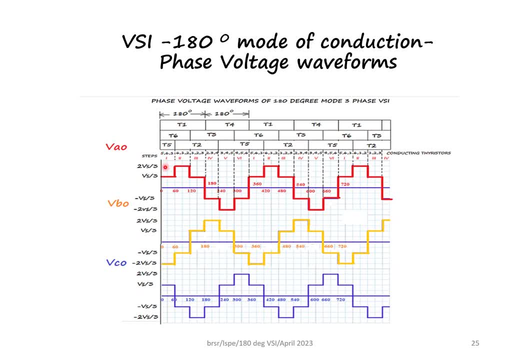 of the voltages, The thyristors which are in operation during 0 to 60 degrees period, is 5,, 6, 1, the very first step we have seen here. it is indicated here In the second step: 0, 60 to 120 degrees. this which is 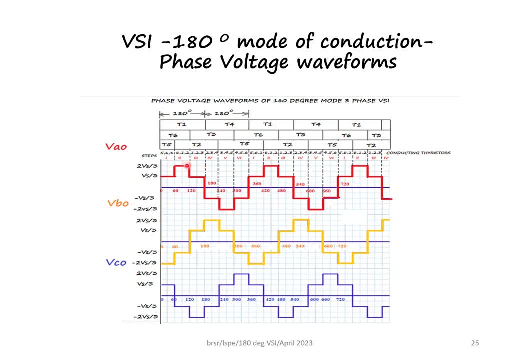 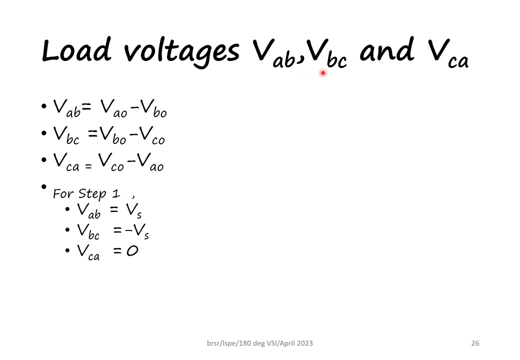 6, 1, 2 are conducting, which is also shown, and the sequence of steps is followed For getting the line voltage waveforms VAB, VBC and BCA. we have to subtract VBO value from VAO to get VAB Load voltages. VAB, VBC, VCA can be derived from VAO, VBO, VCO. like this, VAB is equal to VAO. 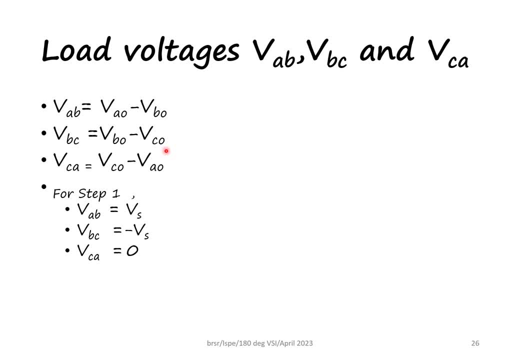 minus VBO. VBC is VBO minus VCO. VCA is VCO minus VCO. VCA is VCO minus VAO. So for the first step, we get VAB, VBC, VCA values as VS minus VCO. We get the line constant value, VAB and VCA values as: 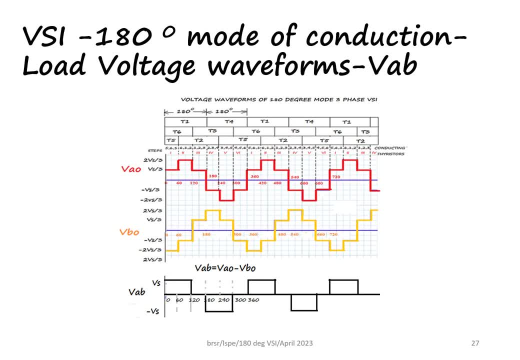 minus Vs and 0 respectively. If we want to get VAB here, we see that we are subtracting BBO from VAO In the first interval, 0 to 60 degrees. the VAB value is Vs by 3 minus of. 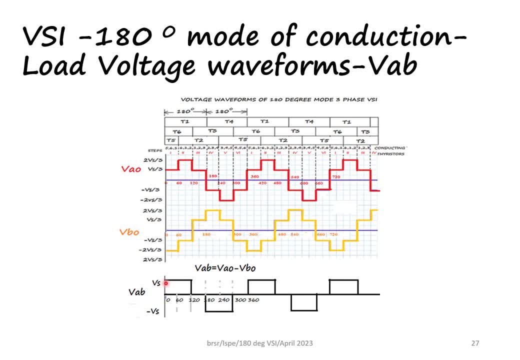 minus 2 Vs by 3.. So we get Vs, and for the next interval, 60 to 120 degrees, the value is 2 Vs by 3, minus of minus Vs by 3, again it becomes Vs. So for each 60 degree interval. 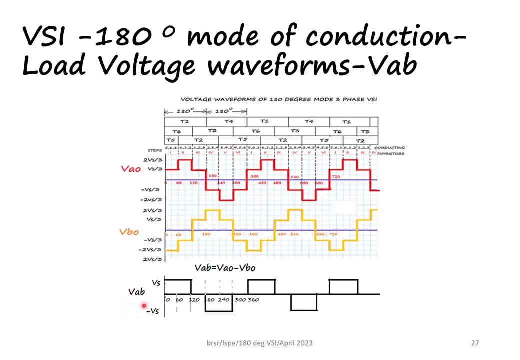 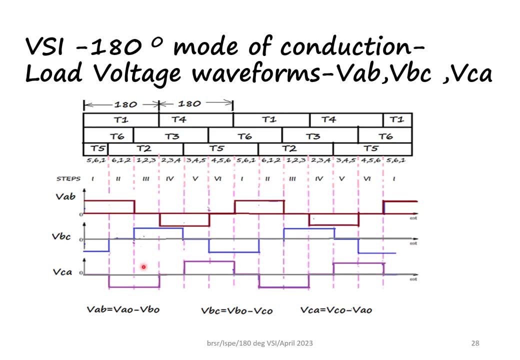 if the value of VBO is subtracted from VAO, we will get VAB, and the line voltage waveform looks like this: The line voltage waveforms VBC and VCA are also shown here. They also follow the same pattern as VAB, as told for the phase voltage. 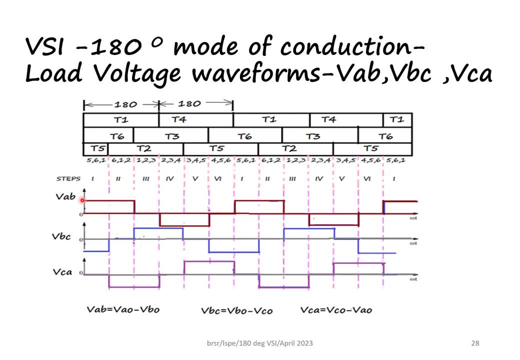 VAB starts with value of Vs at 0,. VBC starts with Vs value at 120 degrees and VCA starts at 240 degrees follows the same pattern. VAB is obtained as VAO minus BBO, VBC as VBO minus BCO. 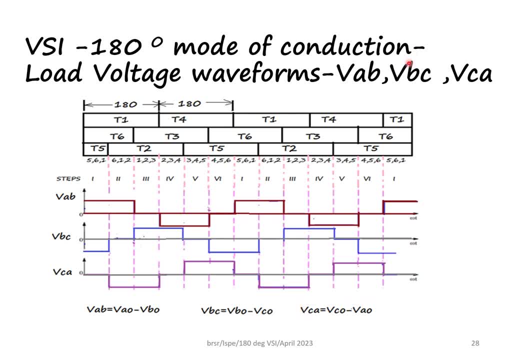 VCA as VCO minus VAO. Hope this explains the operation of a three-phase voltage source inverter in 180 degree mode. Thank you.